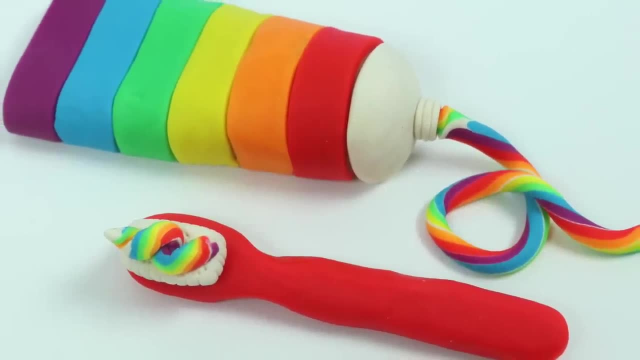 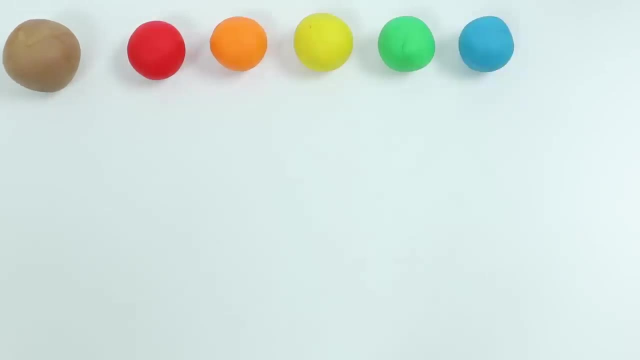 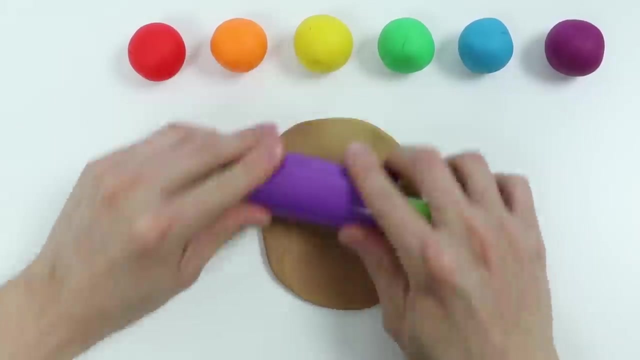 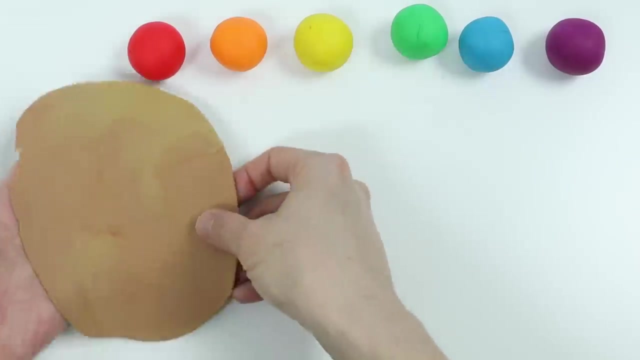 Hey everyone, welcome back to the Awesomer channel. Today we'll be making a rainbow toothbrush and toothpaste with Play-Doh. Alright, let's start by rolling out this brown Play-Doh. Perfect. now let's put this to the side. 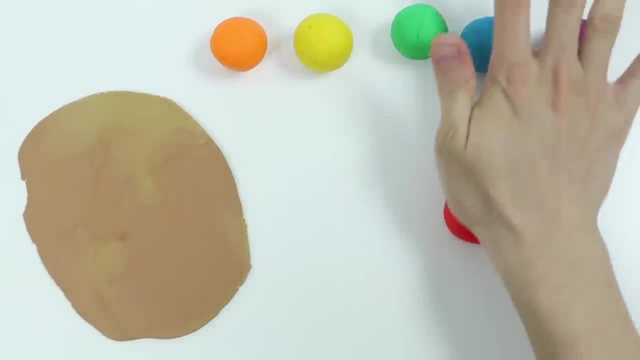 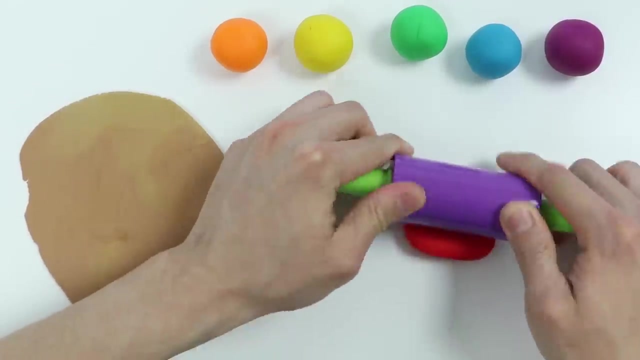 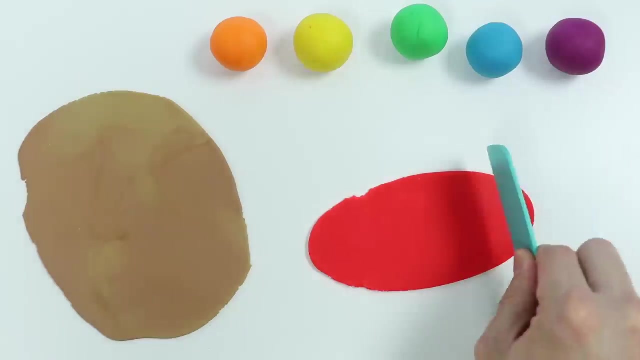 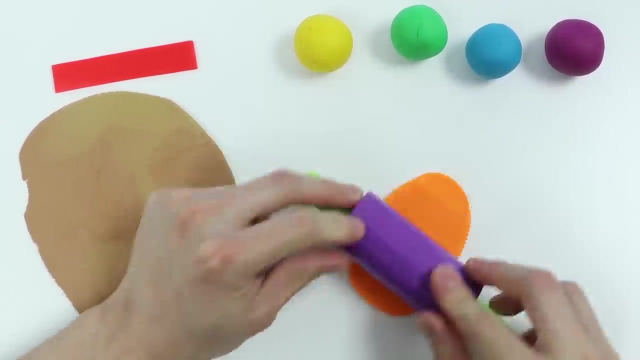 Okay, now let's roll out some red Play-Doh. Alright, now let's make a rectangle shape. Awesome, now let's do the same for the other colors. Let's roll out this orange Play-Doh. Now, let's make a rectangle shape. 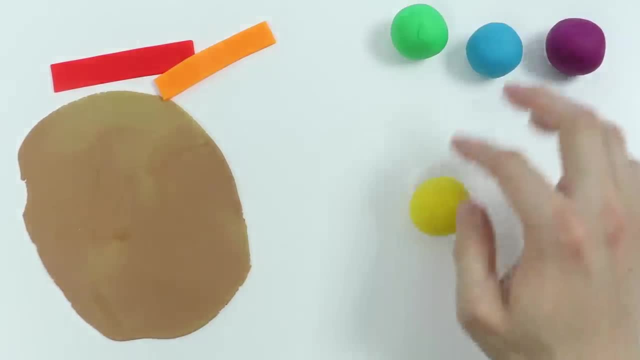 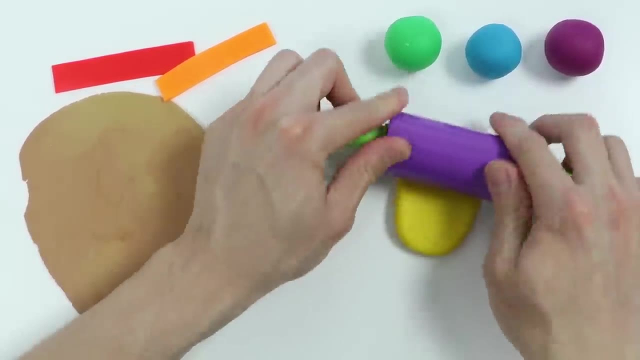 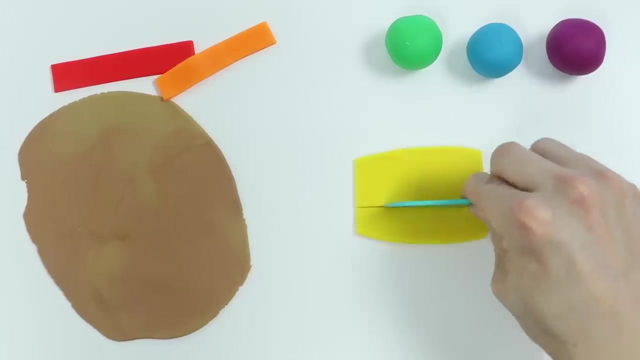 Perfect. now let's make a yellow rectangle. Give me a minute. Awesome. now let's quickly roll out this blue Play-Doh. Now let's quickly make the next two. Now let's make a purple rectangle, and we can move on to our next step. 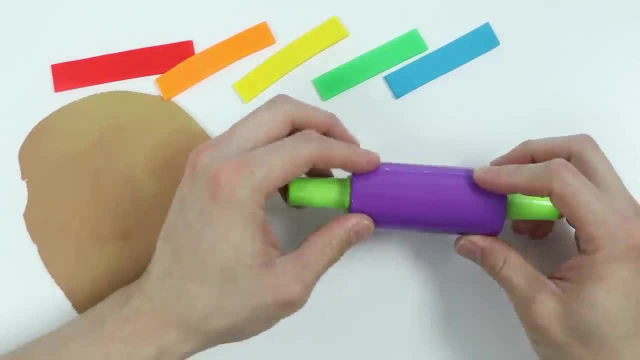 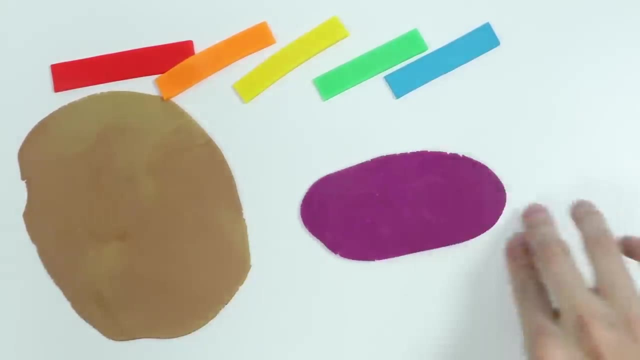 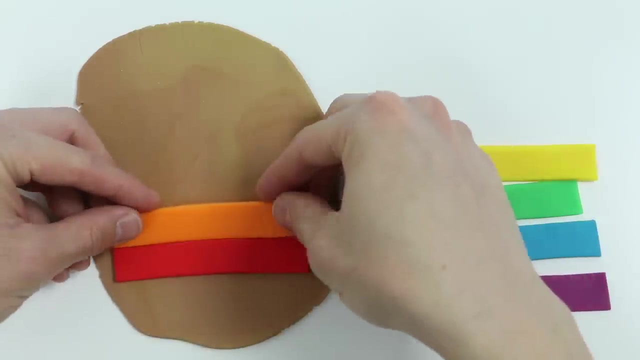 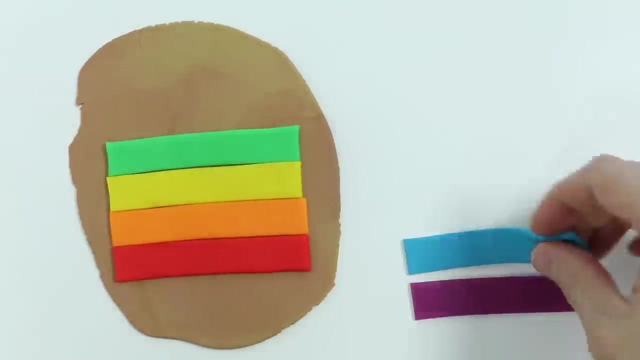 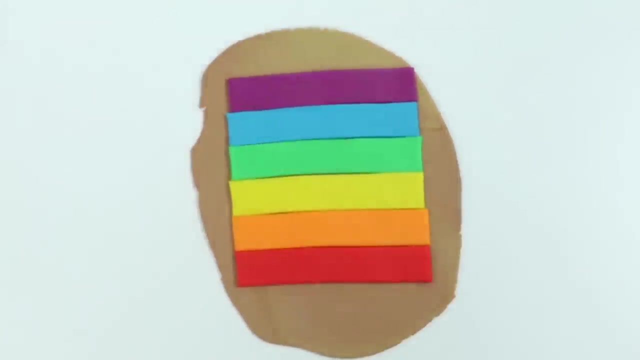 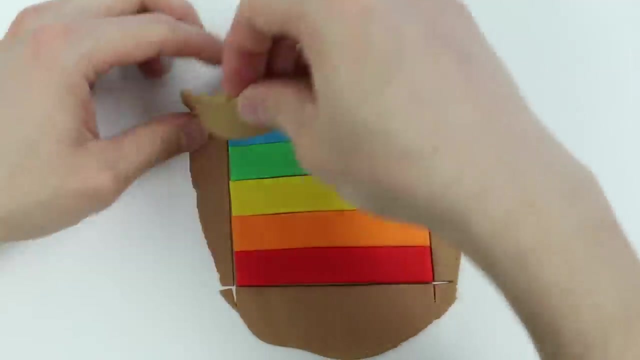 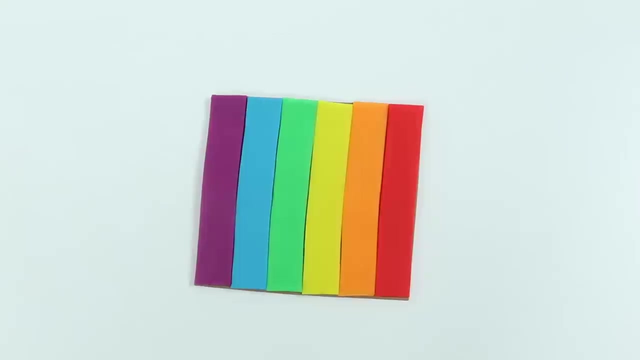 Give me a minute. Perfect. now let's place these strips on top of the brown Play-Doh. Start with red, Orange, Yellow, Green, Blue And purple. Now let's remove all the extra brown Play-Doh. Now let's use the roller to stick the strips on the brown Play-Doh. 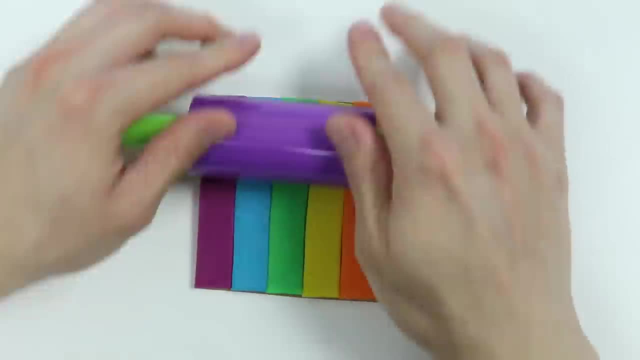 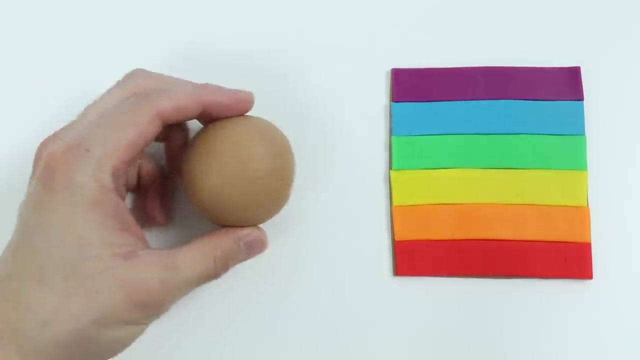 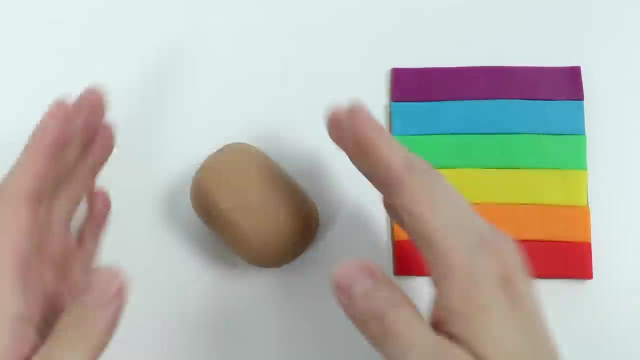 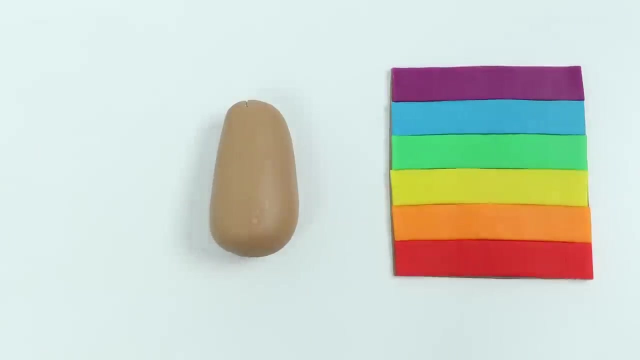 Step 05.. Perfect, now we just make the rainbow toothpaste tube. Alright, now let's roll out another ball of brown play-Doh. Give me a minute, Step 06.. Step 07.. Step 08.. electronic loud. 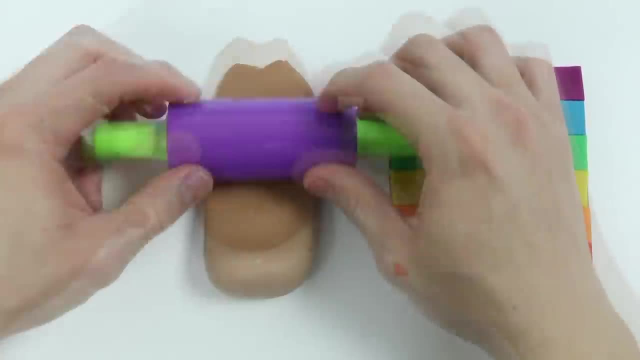 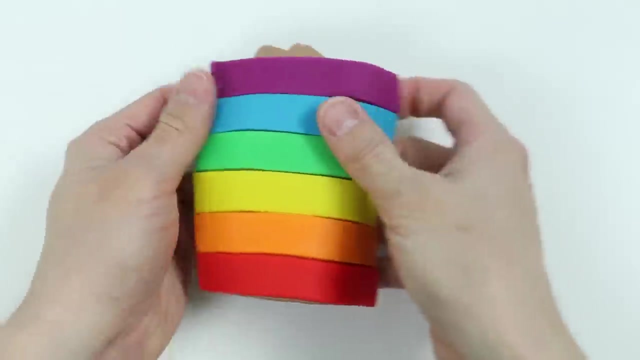 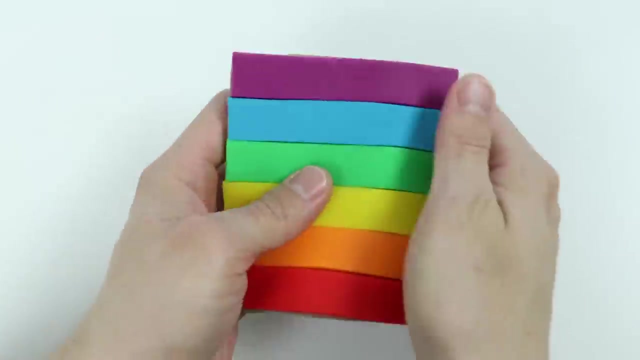 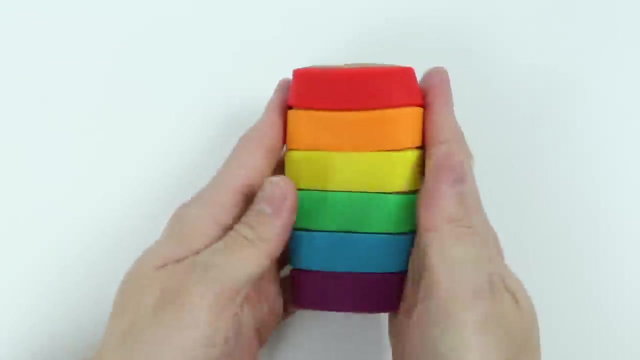 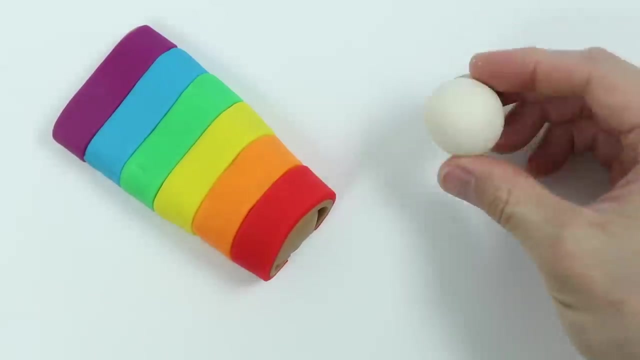 Esta la All right. now let's wrap our rainbow tube around the brown Play-Doh. Cut this extra Play-Doh, clean this up. awesome, Here's our rainbow toothpaste tube. Now let's finish it up by making the cap area. 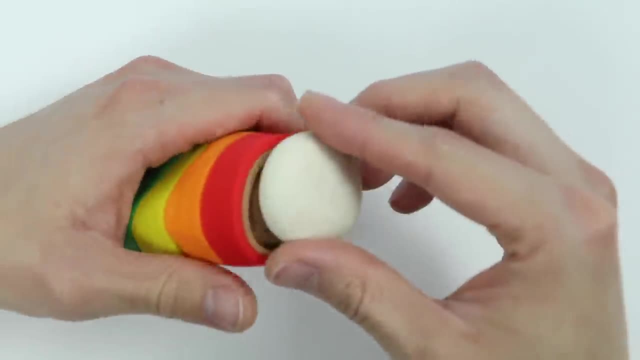 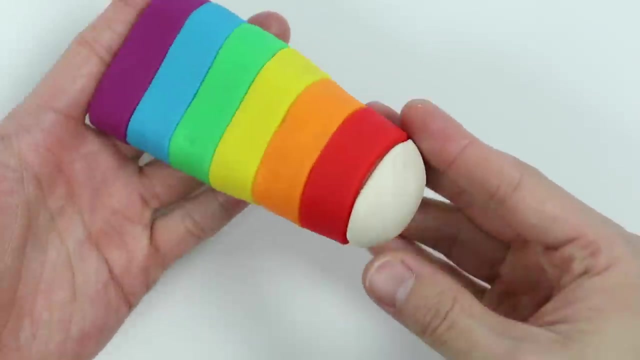 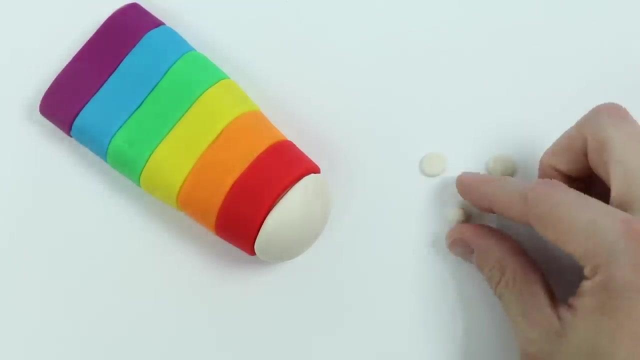 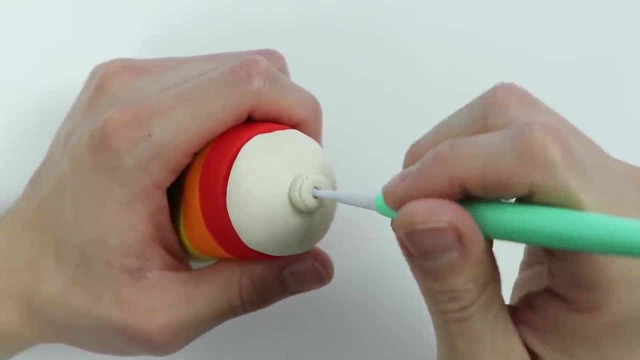 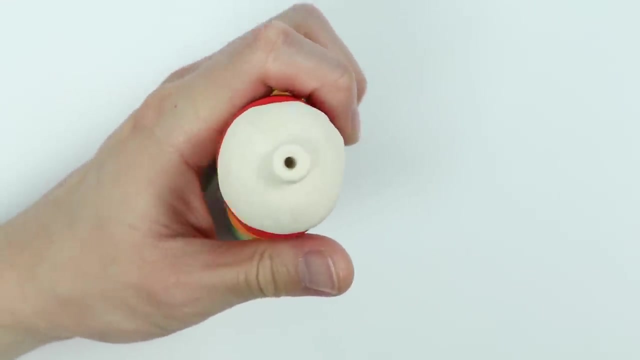 Use some white Play-Doh. All right, we're almost finished. Let's add a few more details. Use some more white Play-Doh. We're almost done. Perfect, Awesome. We just made our rainbow toothpaste tube. Now let's make some toothpaste. 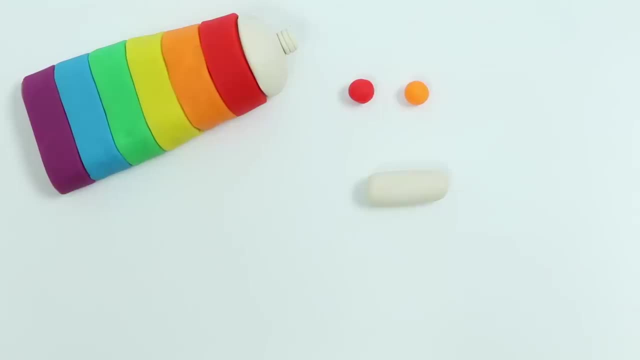 We'll need some more white playdough and a few other colors. Let's start by rolling this ball of red playdough. This is the shape we want. Let's do the same for the other colors. Now let's attach all of our rainbow colors onto our white playdough. 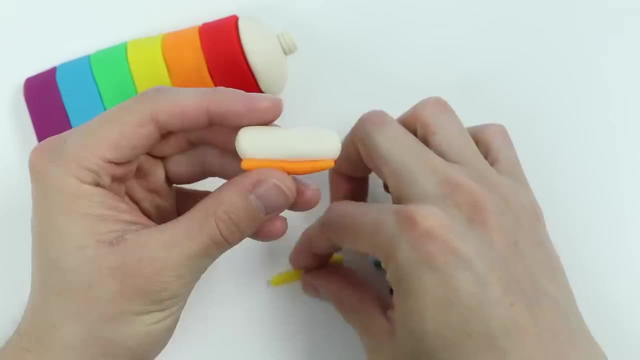 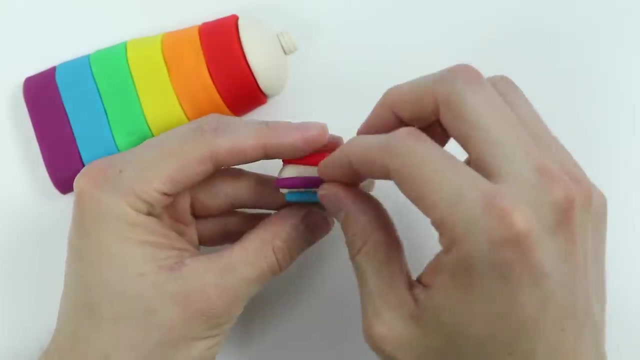 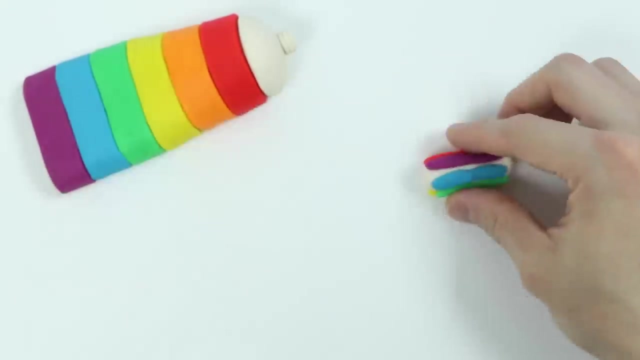 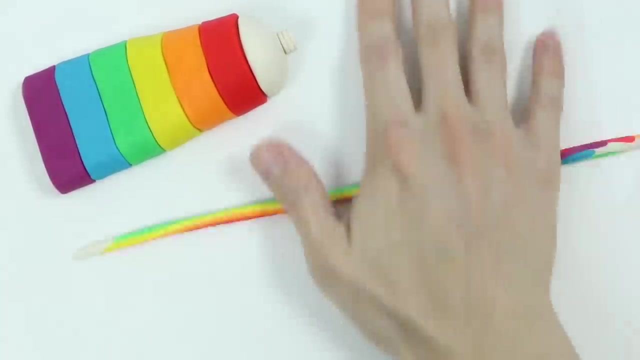 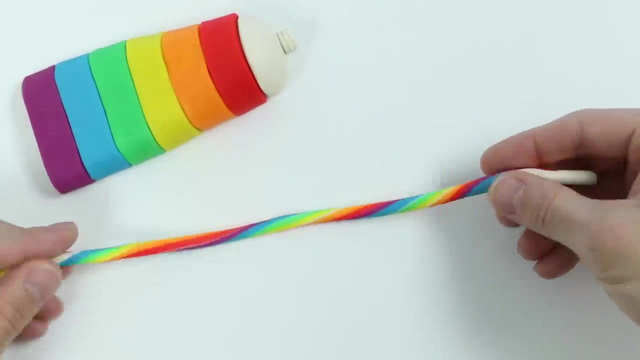 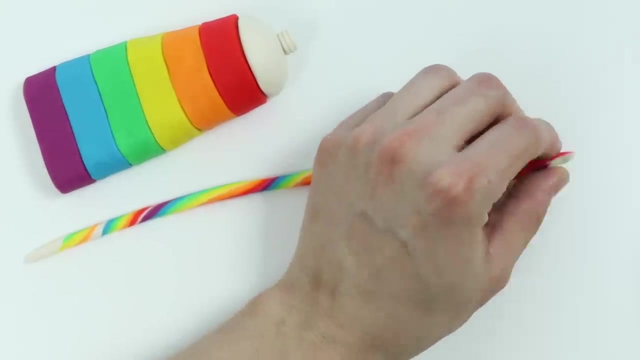 Give me a minute, Okay. Okay, now let's roll this out. That looks pretty good. Let's make it a little better by twisting it. Now, this is a pretty looking toothpaste. Let's cut the end right here and attach it to the tube.